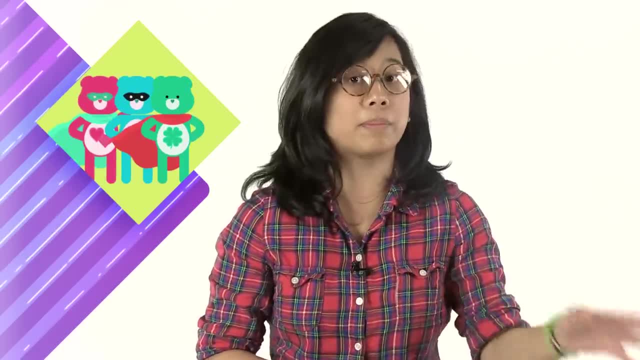 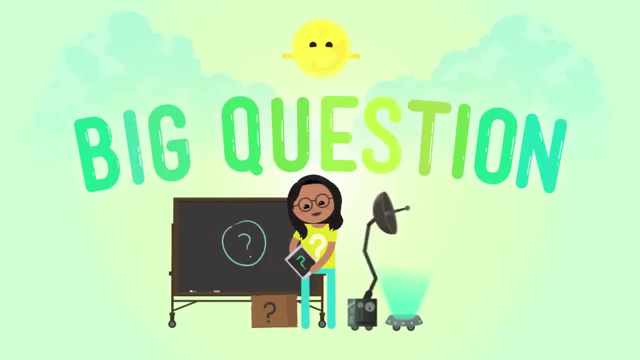 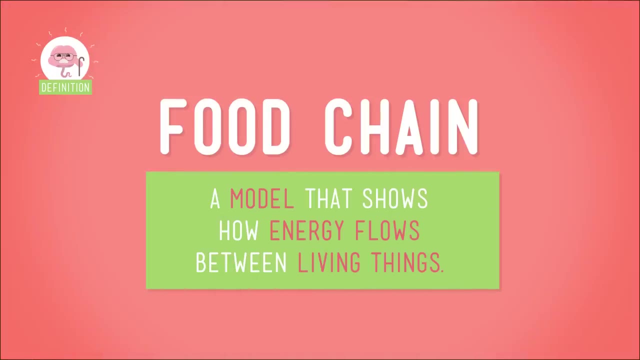 and except for the occasional video game monster and maybe the odd bear, nothing tries to eat us. But what is a food chain exactly? A food chain is a model that shows how energy flows between living things. You can think of animals and plants in the same food chain as all living in the same neighborhood. which. 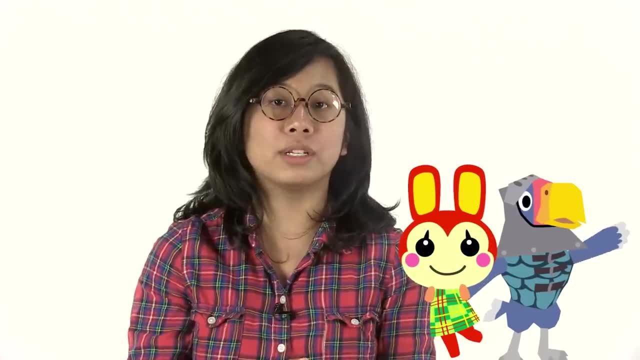 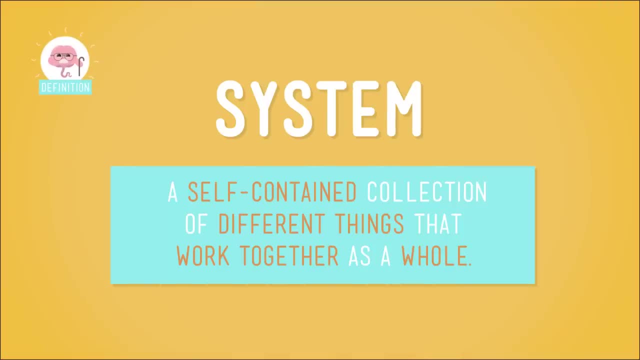 scientists call a habitat, and they all have a job to do, interacting with each other day in and day out. Together they form a kind of system, a self-contained collection of different things that all work together as a whole, And they also interact with the non-living. 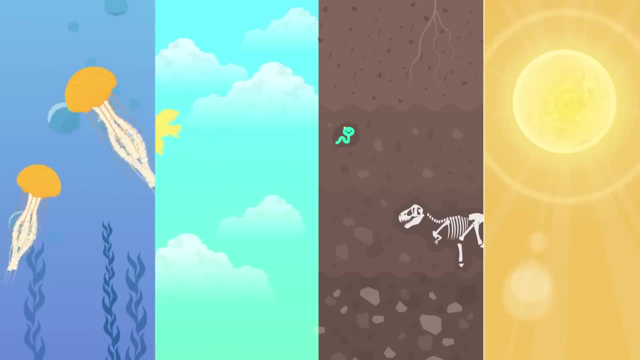 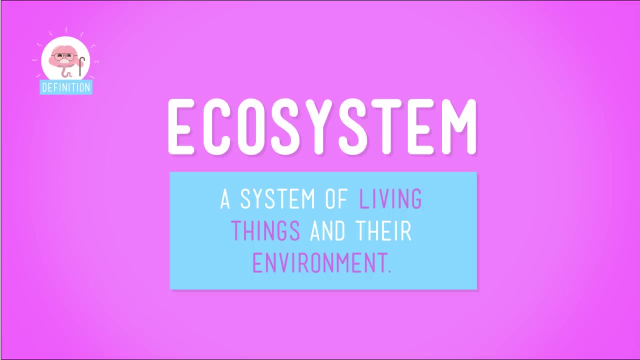 stuff around them, like the water, the air, the ground, the air, the air, the air, the ground and the sun. Put it all together and what do you get? A special system called an ecosystem and food chains. show us what eats what in an ecosystem. Now, everything. 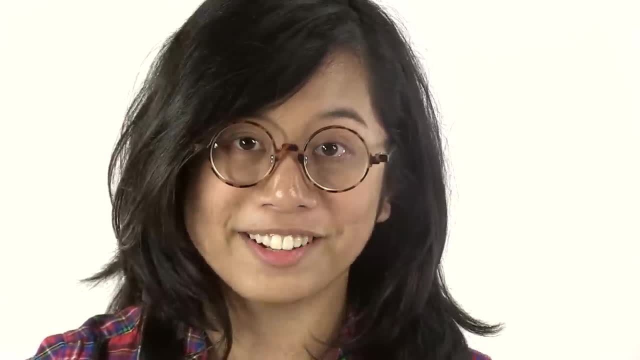 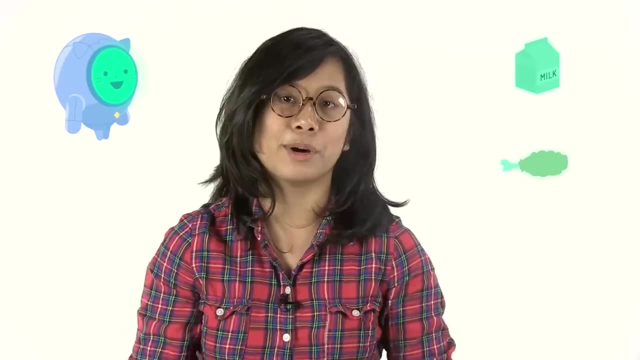 that's alive is in a food chain, including you, my friend, And actually most living things are in more than one food chain, depending on what or who they're munching on at the moment. I mean, you don't eat the same thing for dinner every night, do you? Didn't think? 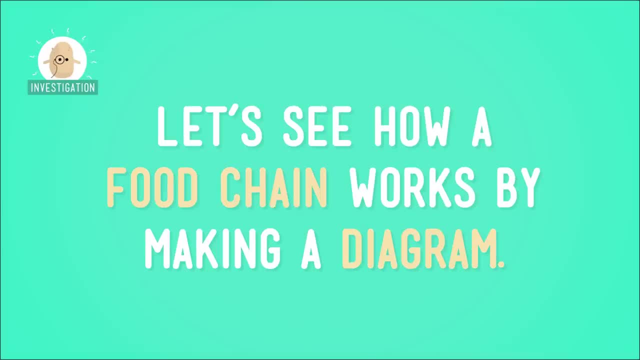 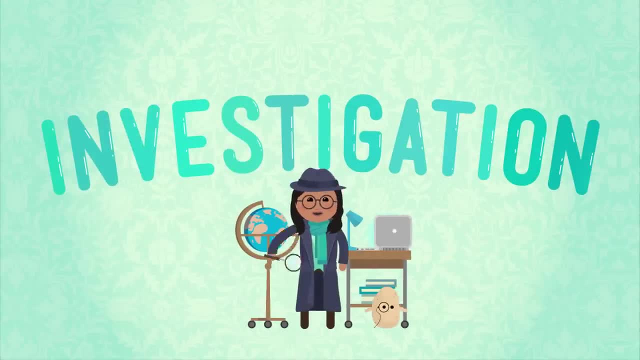 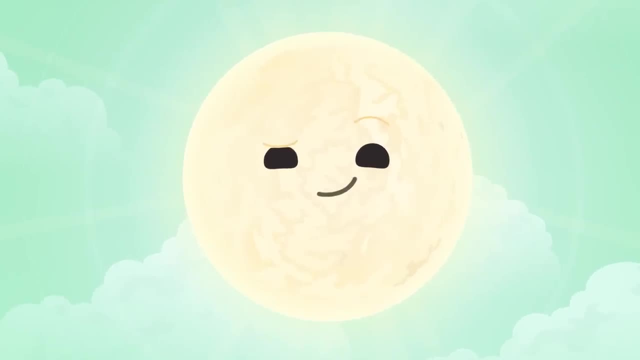 interactions happen in nature. First, all of the energy that's in a food chain starts with the sun. I can't stress that enough. people, Plants- take the energy from the sun's rays and change it into chemical energy. So when a nice patch of lush green grass starts to grow, it's capturing. some of the energy from the sun to do it. Then, when an animal like a rabbit wanders by and nibbles on that grass, the energy from the plant is transferred to the sun. Now, if a hungry hawk decides that the rabbit would make a yummy supper, then the energy 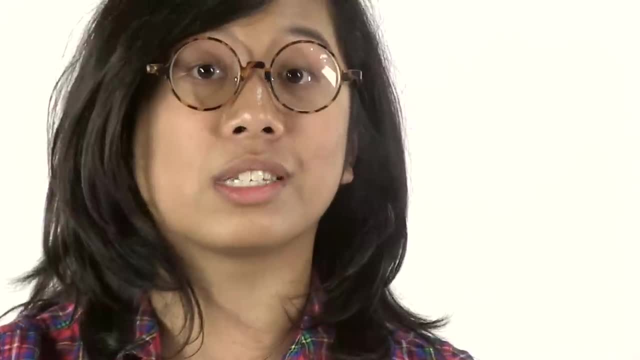 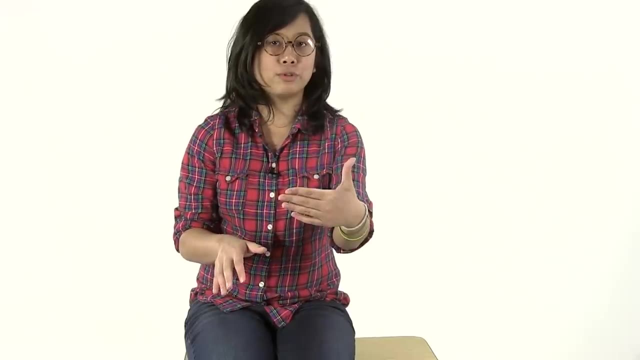 from the rabbit is transferred to the hawk, And in this ecosystem, nothing is large or brave enough to take on the hawk. I mean, just look at her. So we've hit the top of the food chain and we've just made a nifty model of it.